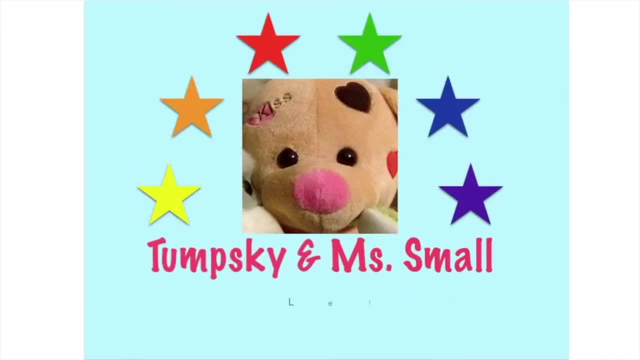 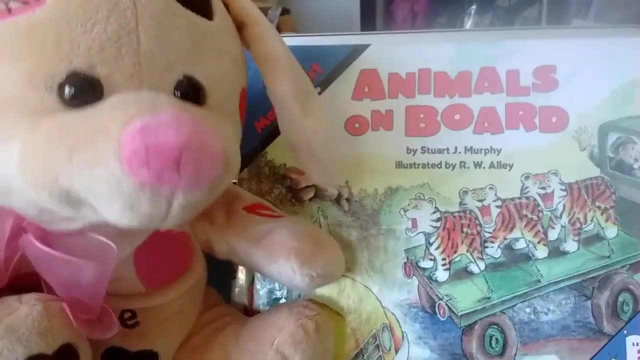 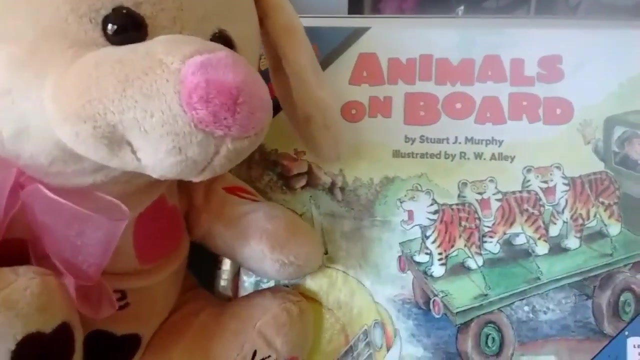 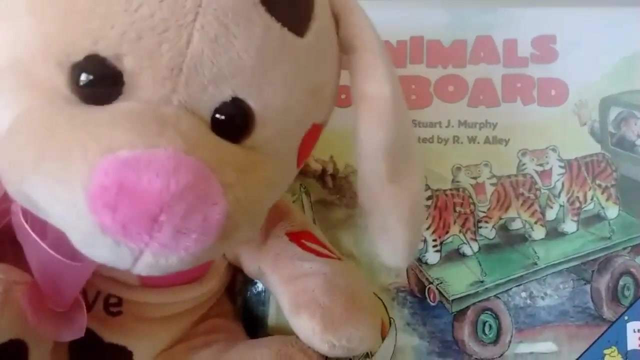 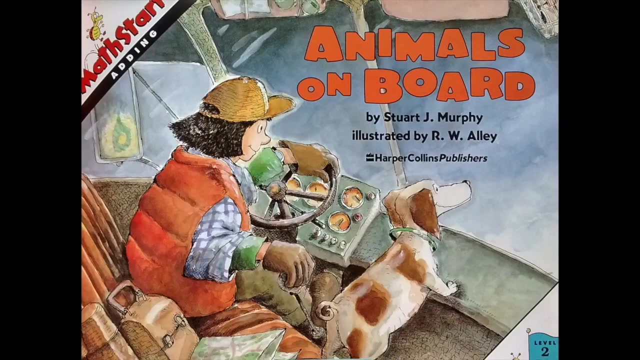 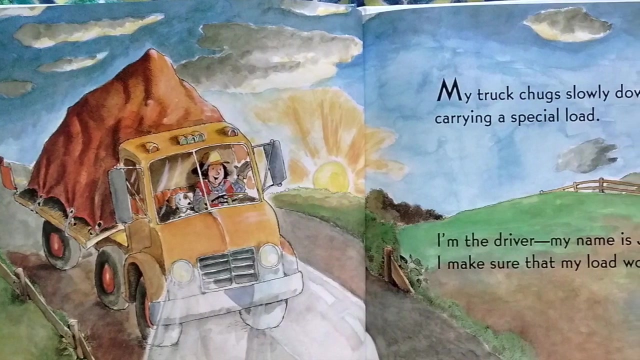 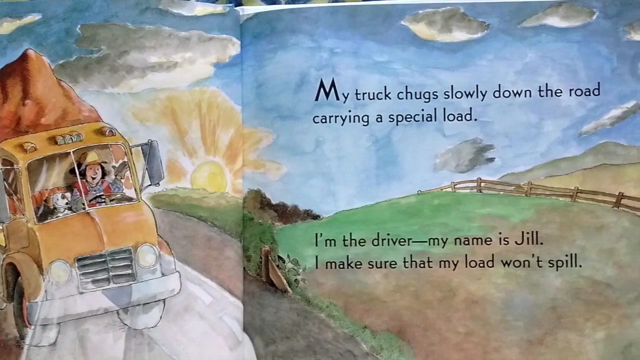 This book is called Animals on Board and it is by Stuart Murphy and pictures are by RW Alley. It's a math book. You're going to like this one. Sit tight, friends. My truck chugs slowly down the road carrying a special load. I'm the driver. My name is Jill. I make sure that my load won't spill. 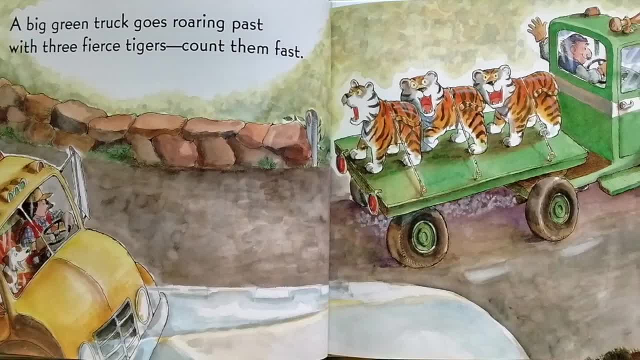 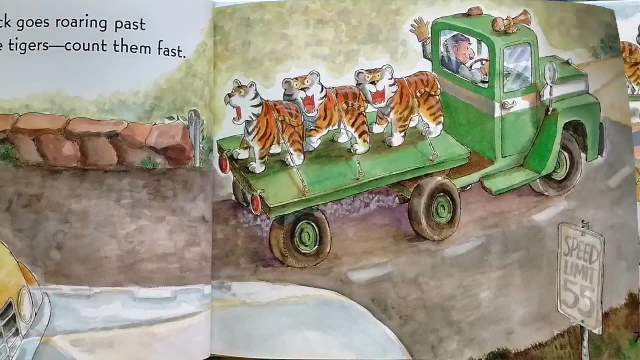 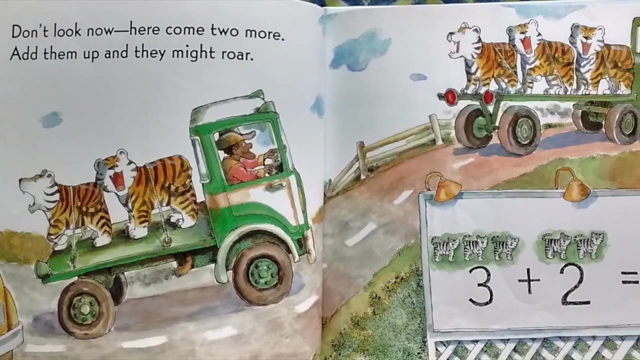 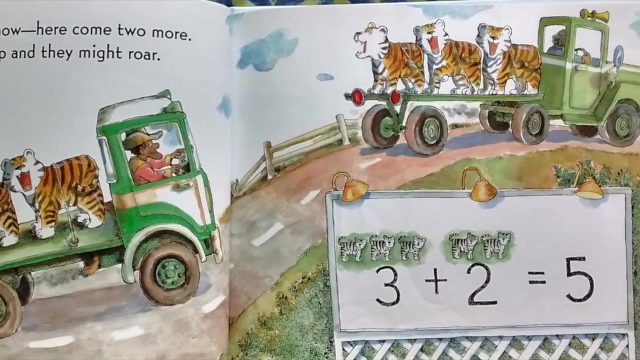 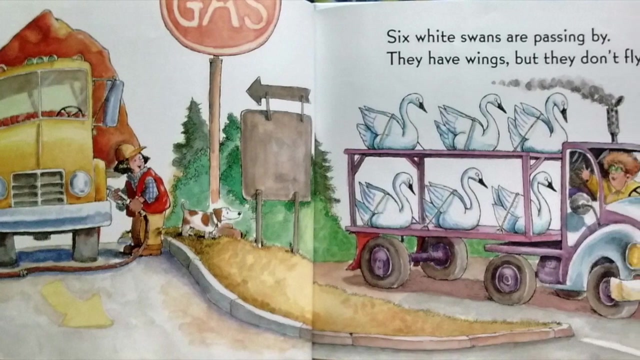 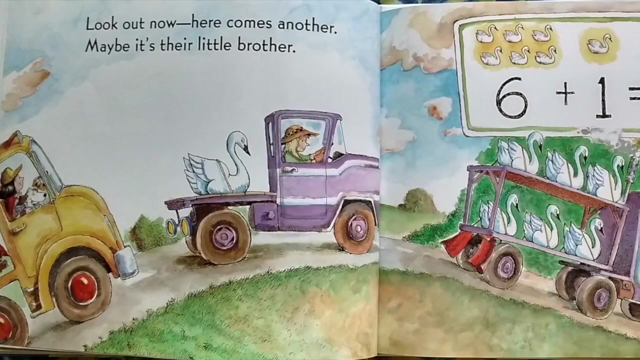 A big green truck goes roaring past with three fierce tigers. Count them fast, Don't look. now Here come two more. Add them up and they might roar. Three plus two equals five. Six white swans are passing by, They have wings, but they don't fly. Look out. now Here comes another. 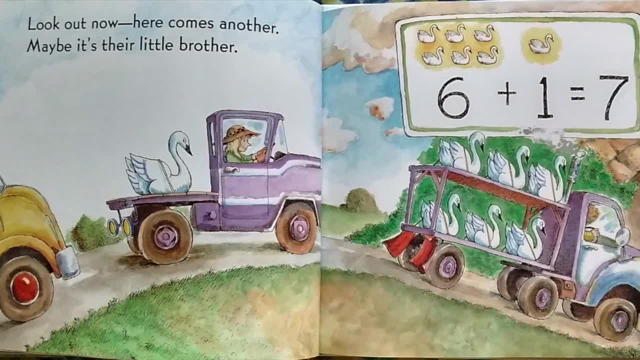 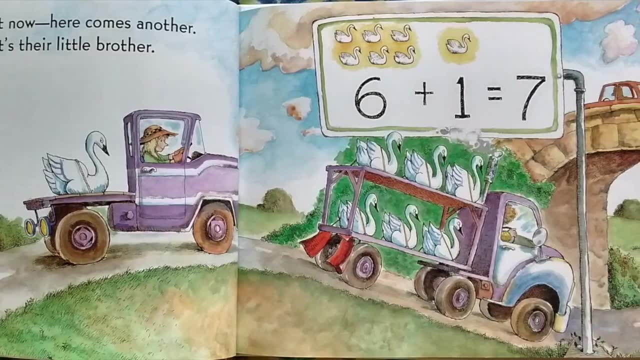 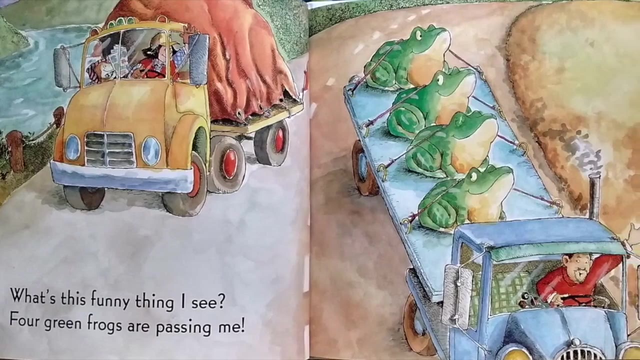 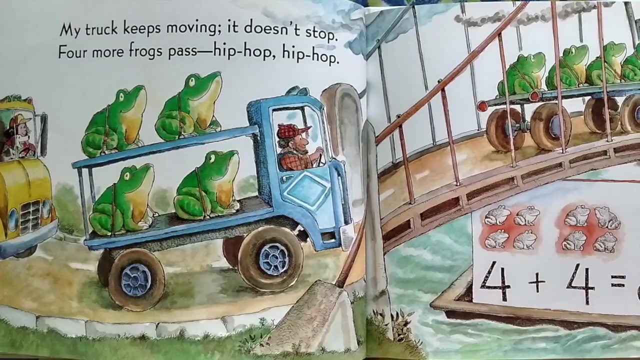 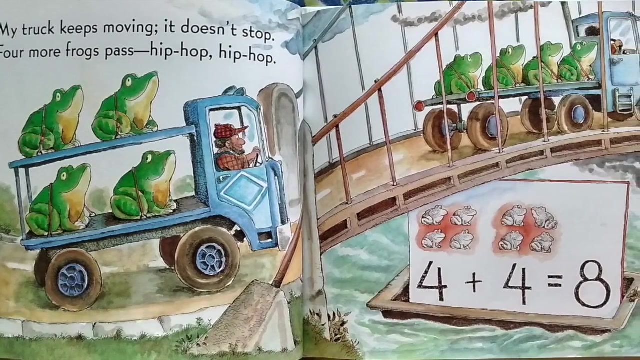 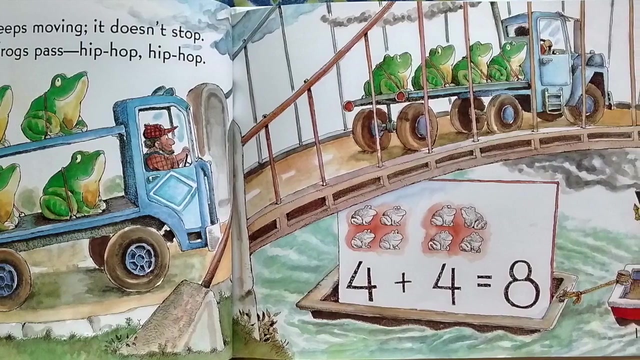 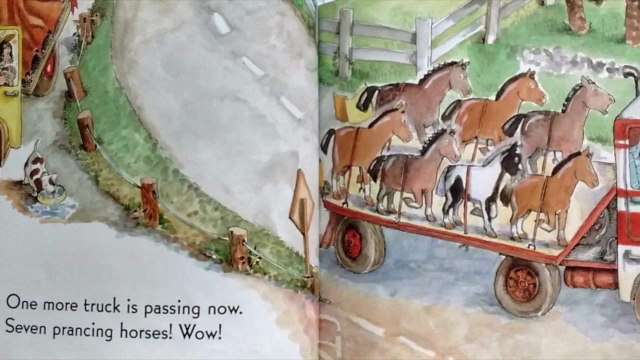 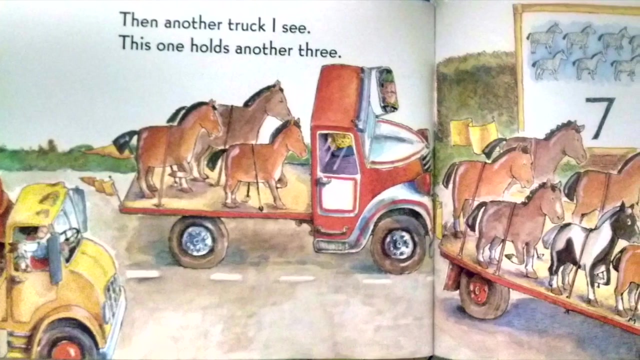 maybe it's their little brother. six plus one equals seven. what's this funny thing? I see four green frogs are passing me. my truck keeps moving, it doesn't stop. four more frogs pass, hip hop, hip hop. four plus four equals eight. one more truck is passing now, seven prancing horses. Wow, then another truck. I see. this one holds. 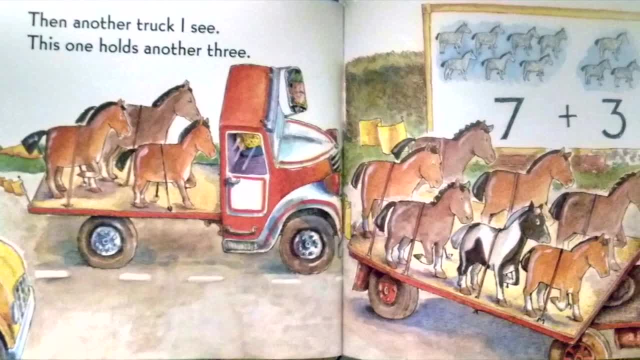 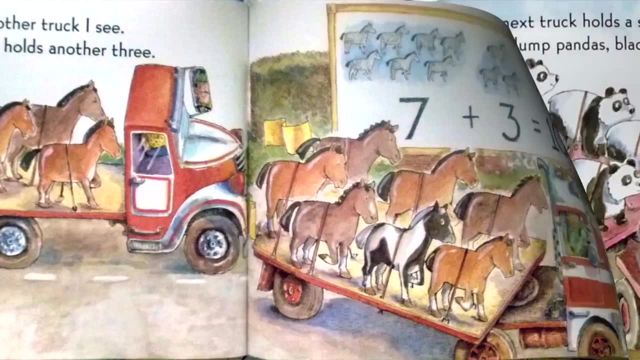 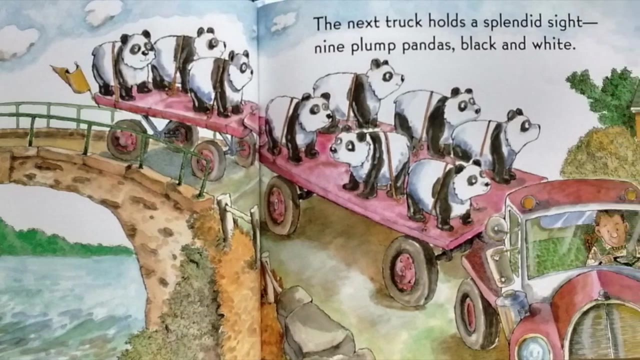 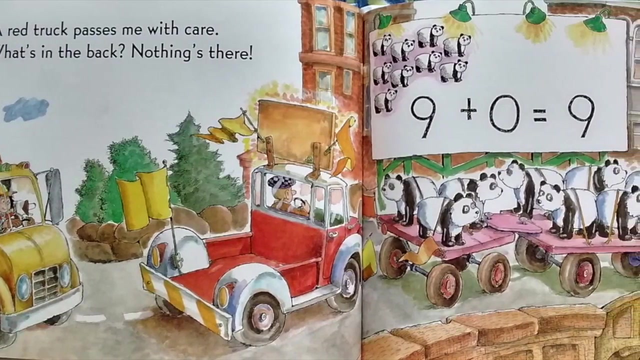 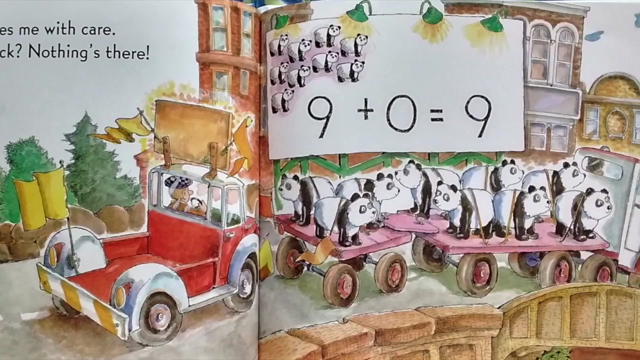 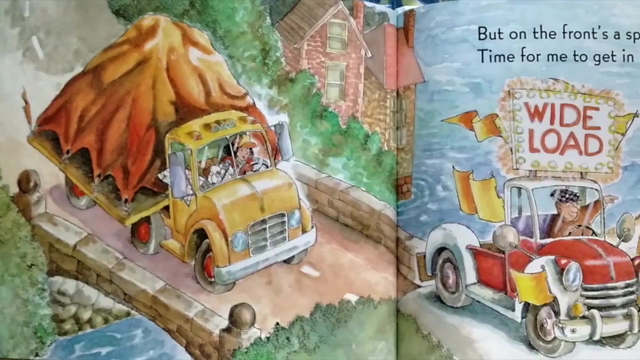 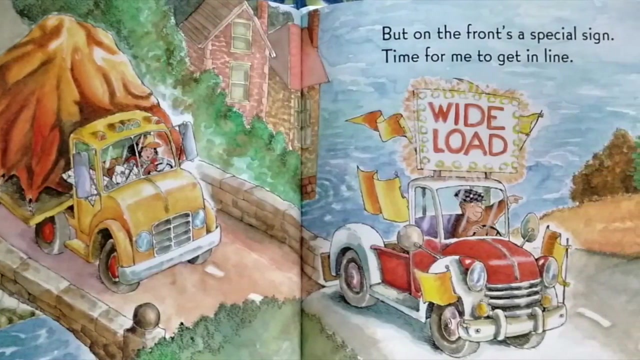 another three plus three equals ten. the next truck holds a splendid sight: nine plump pandas, black and white. a red truck passes me with care. what's in the back? nothing is there. nine plus zero is nine, but on the front, the special sign. time for me to get in line. wide load the next. 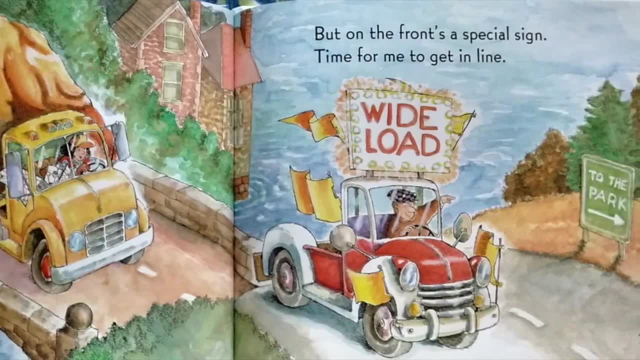 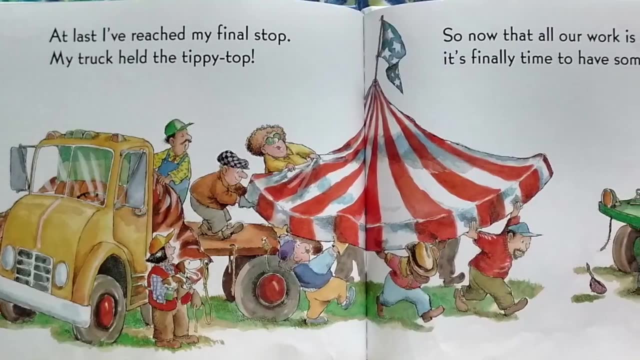 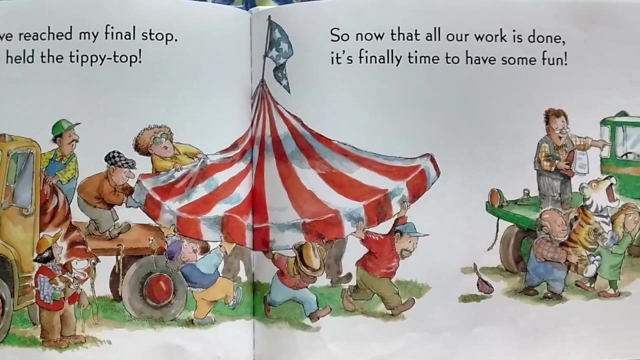 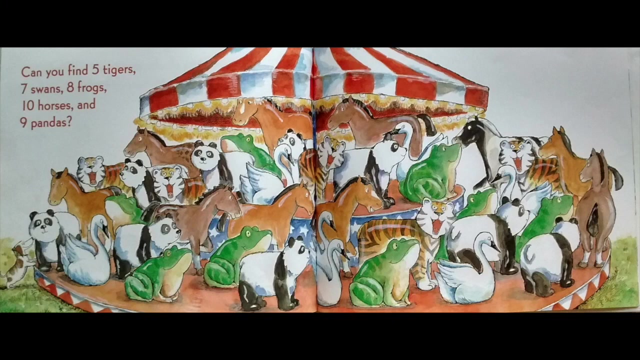 sign says to the park: at last I've reached my final stop. my truck held the tippy top, so now that all our work is done, it's time to get eavesdropping on the road. finally time to have some fun. Can you find five tigers? How about seven swans? 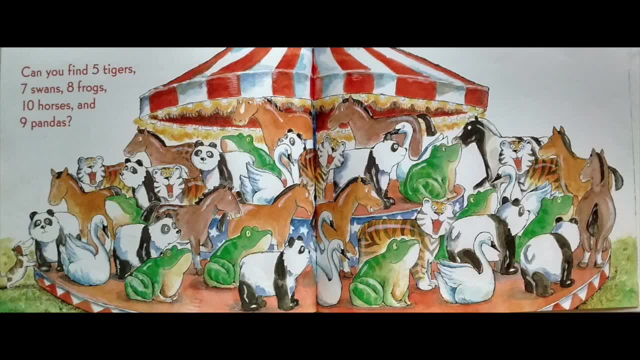 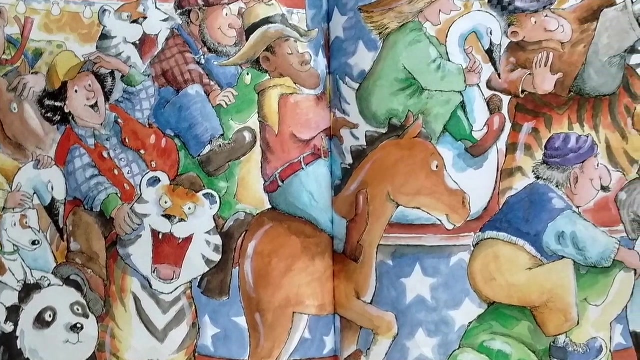 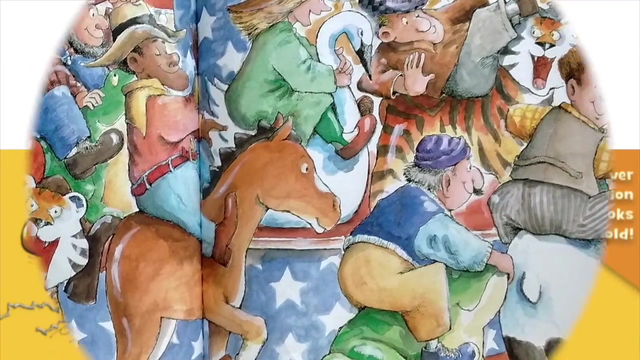 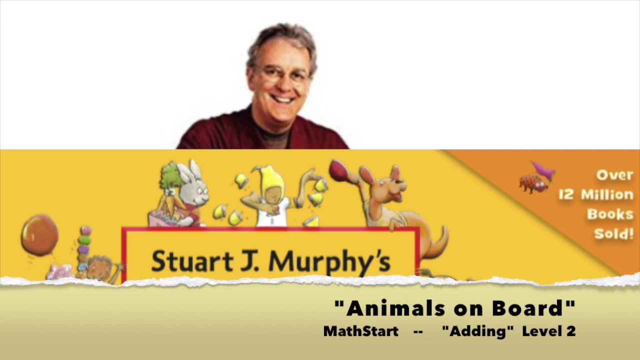 Eight frogs, ten horses and nine pandas. After all that hard work, everyone's having fun now. Thanks for watching, friends. That's the end. Look for more of Stuart J Murphy's books from Math Start. Not only do you get a story, 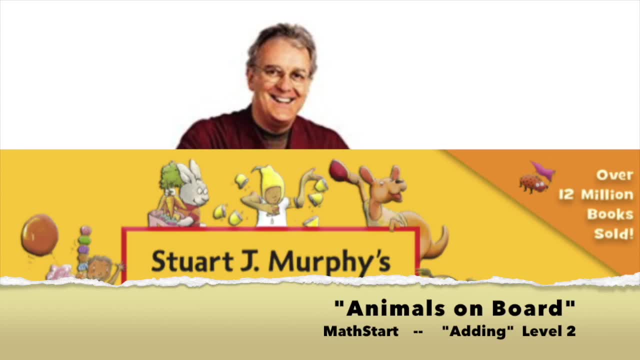 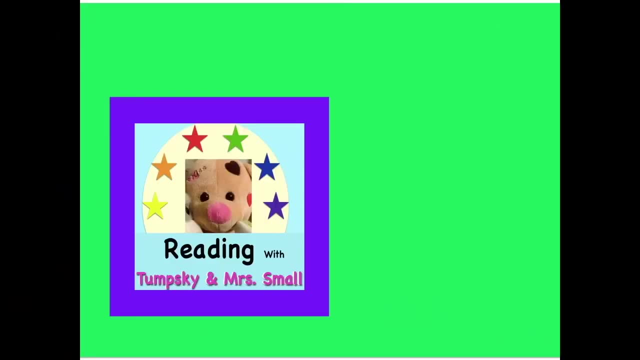 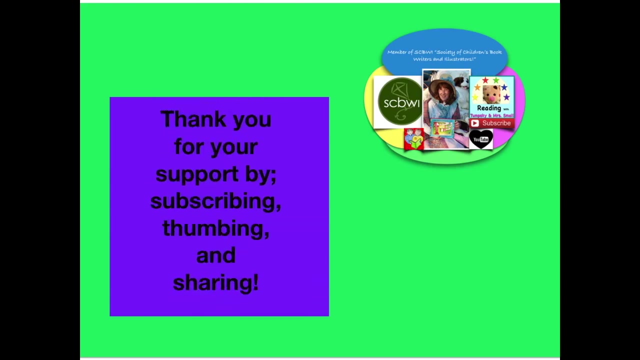 but you also get some math. See, math can be fun. See what other things you can count near you. Well, we're done. So if you want to learn more about math, click on the link in the video description. It is a great way to learn math in a really simple way. 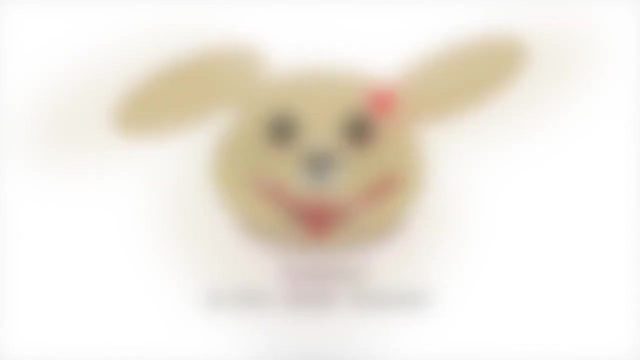 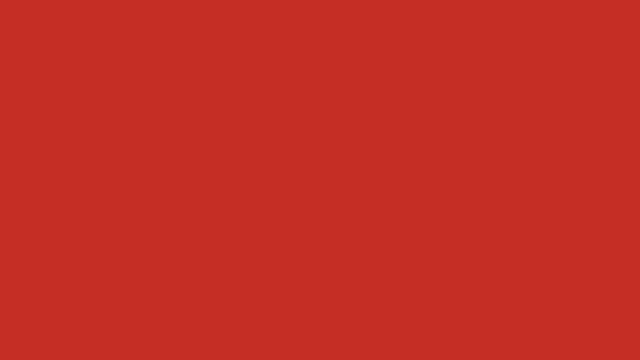 We've got two shows: refresher andenglish.